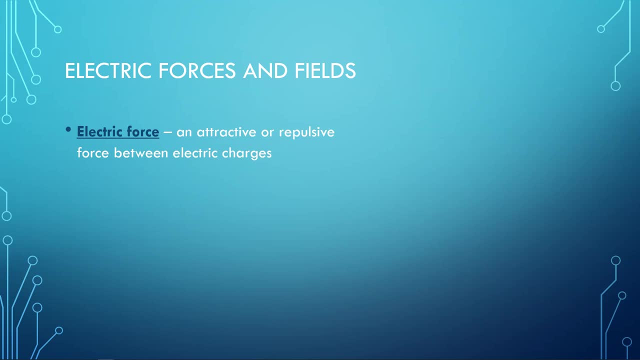 but sometimes they have a positive or a negative charge due to too many or too few electrons. An electron is an extremely tiny particle with a negative charge. An electric force is a force which is a push or a pull that is between objects or particles that are not neutral. 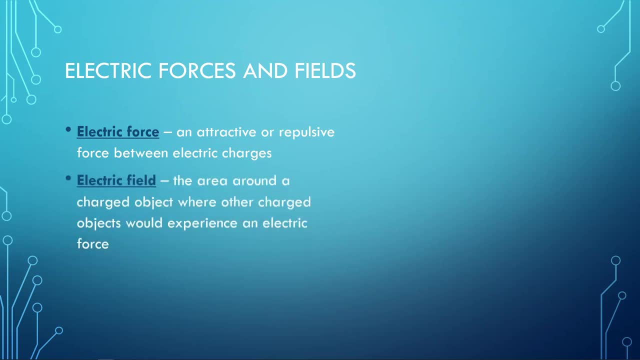 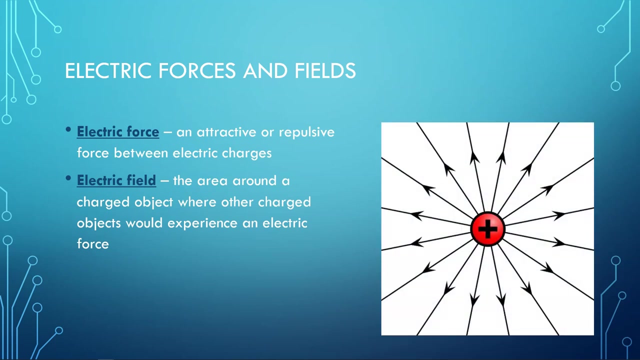 so either positive or negative. An electric field is the area around a charged object or particle where other charged objects or particles would experience an electrical force, a push or a pull. This image shows what the electric field around a charged object might look like. The lines and arrows represent 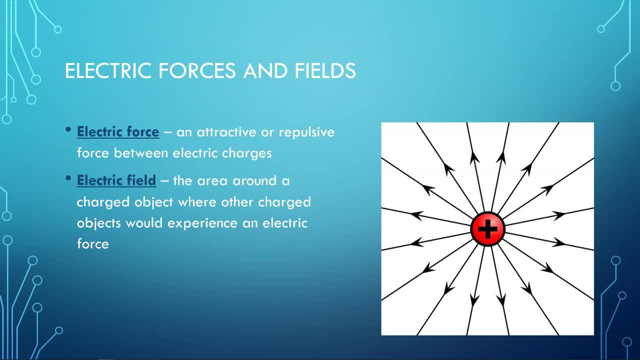 the direction that positively charged objects move, which is positive to negative. Now keep in mind those lines that you see aren't actually there in real life. They are invisible. The electric field lines are drawn there to show the area around this charged object where another charged 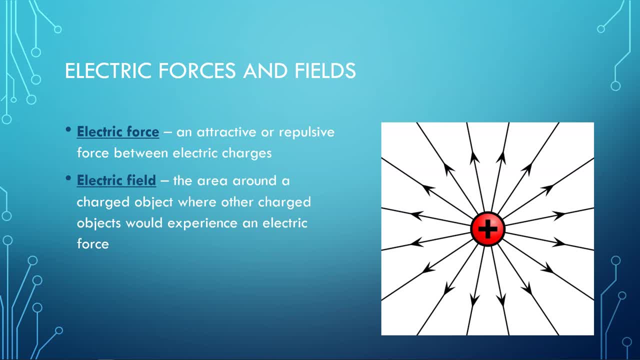 object would experience a push or pull when it got close enough. Different areas of an electric field have different levels of strength. The strongest area of an electric field is at its center, close to the charged object. Any charged objects in this strongest area would be highly. 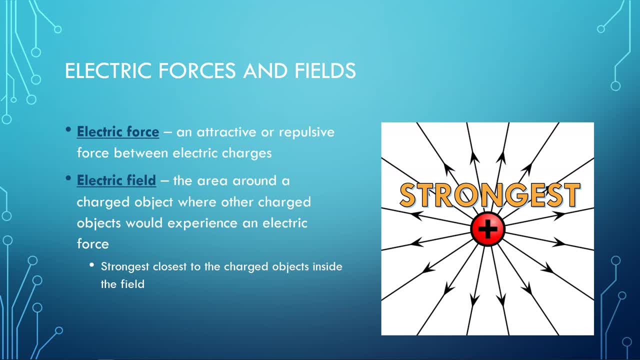 affected either with a strong push or a strong pull. However, the further and further you get from the center of an electric field, the stronger the field is, The weaker it is. Get far enough away and you'll be out of the electric field completely Charged. 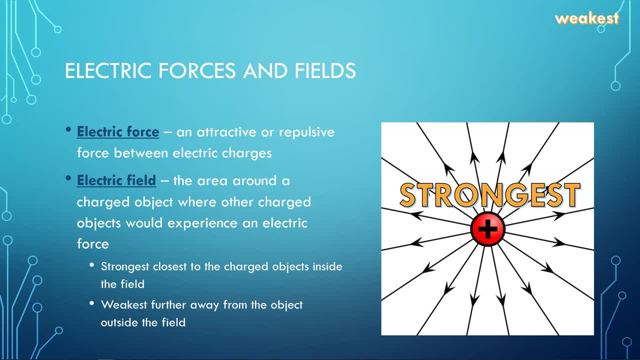 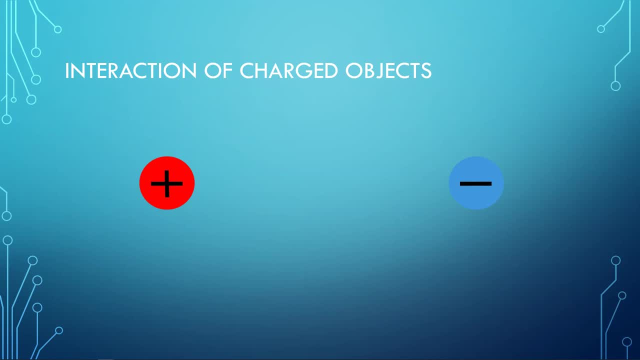 objects far from the center are less likely to be pushed or pulled, since the field is so much weaker. Charged objects interact with each other in unique ways depending on if the charges are opposite or the same. When charged particles are opposite, they attract one another or pull toward. 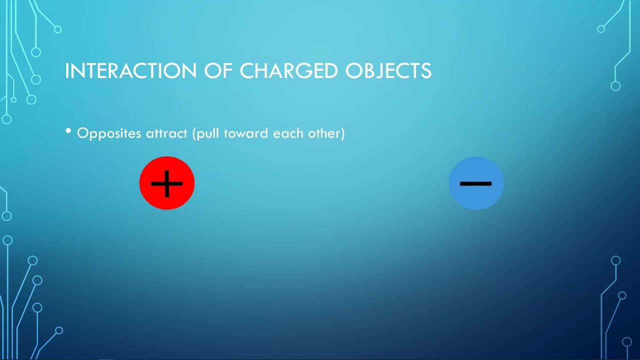 each other. Here we have a charge that is opposite to the charge that is pulled toward each other. Here we have two balls. The one on the left has a positive charge and the one on the right has a negative charge. Opposite charges are attracted to one another, so if these charged balls are close,